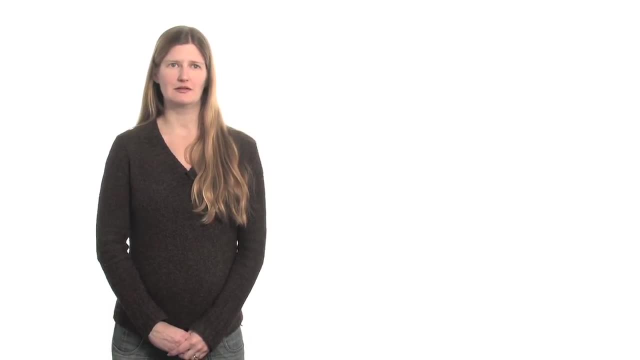 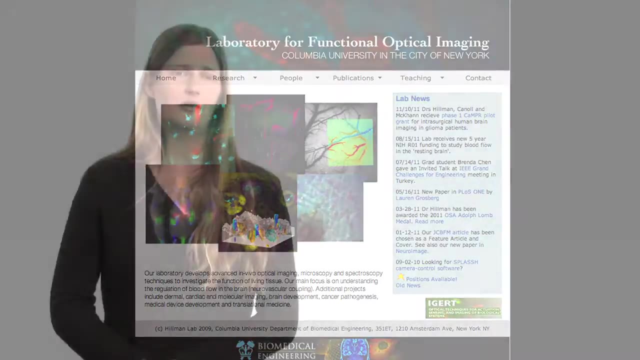 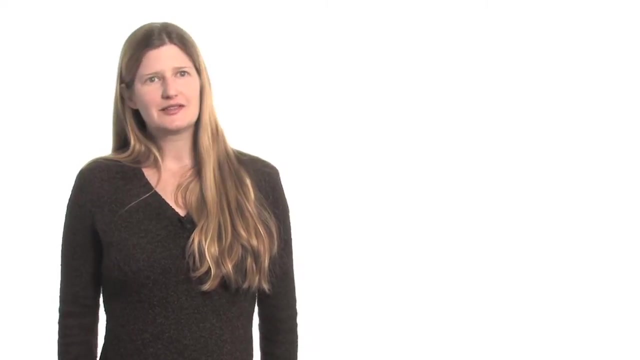 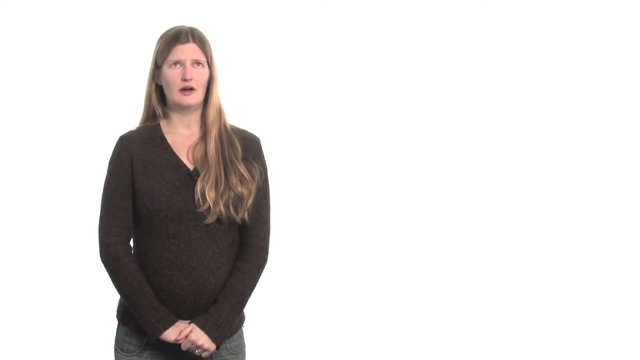 in developing and applying optical techniques for imaging living things. We're primarily driven by this question about the brain, but a lot of our techniques now have spanned out into other areas like skin cancer and other kinds of cancers and gastrointestinal tissues and heart activity- things like that. The work that we're doing could have a high impact. 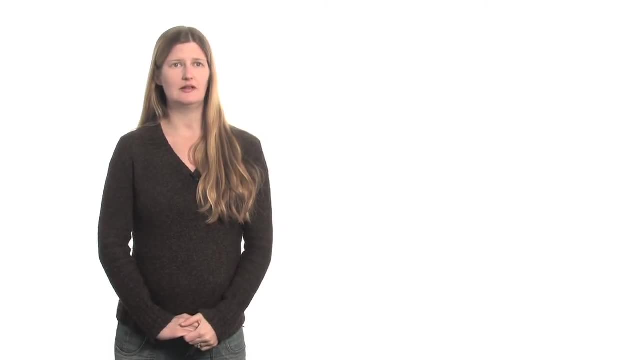 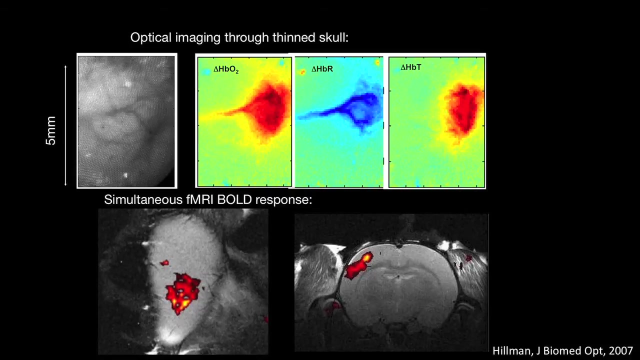 on understanding functional brain imaging modalities that are used in humans, like functional MRI and even PET studies, And so really being able to provide the information about what those techniques are actually measuring and assist with interpretation of that data and guide imaging paradigms to fit better to the sorts of physiology that's. 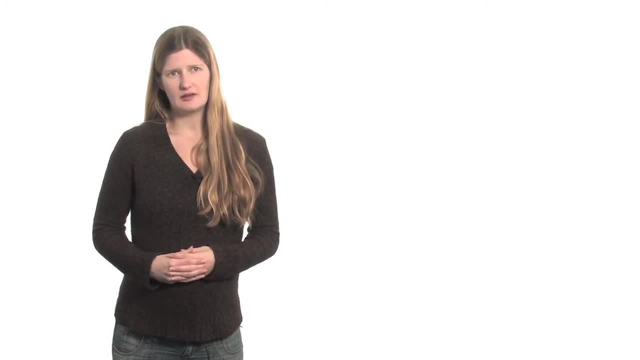 going on could have a real impact. Also, the techniques that we're developing generally. so far we've done a lot of stuff in sort of normal models, but they can be readily applied to new models of disease. We've been working recently looking at development in the brain. 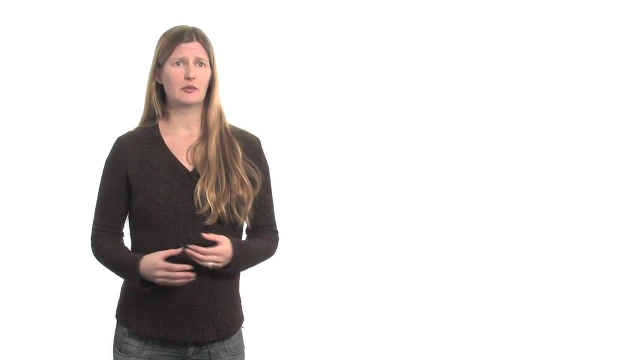 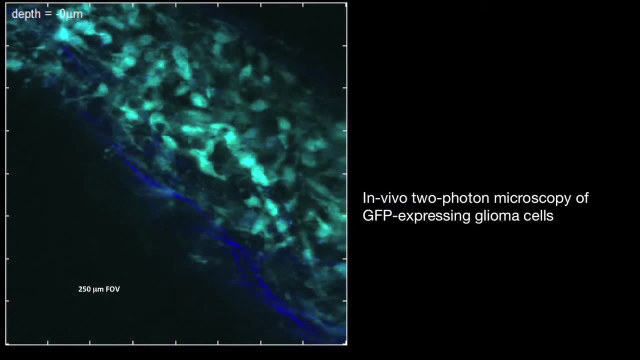 and also recently looking at glioma and how glioma develops, And so if we can provide answers about how glioma cells migrate through the brain and maybe even use our systems to look at potential therapies and say, well, how do they affect the way that glioma cells migrate through the brain? 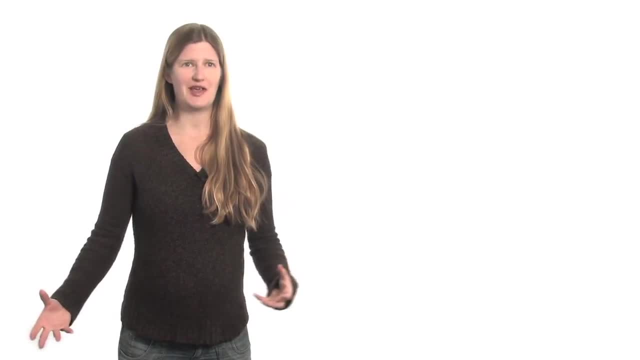 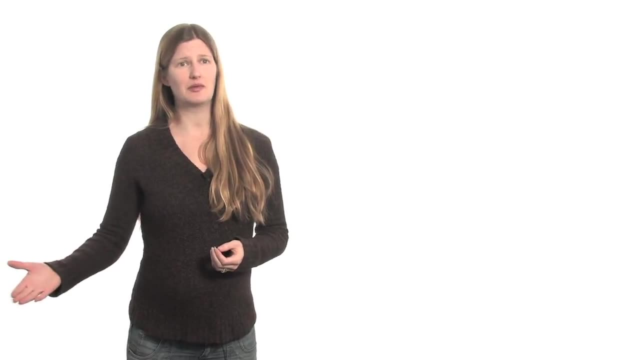 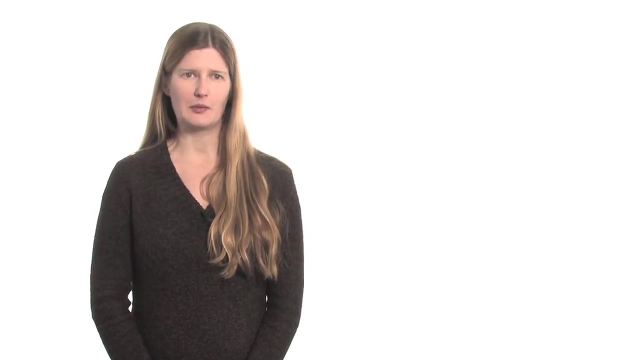 How does this treatment work and why does it change the outcome in a human? We've been able to provide something that can really be directly applied to human treatment, but without our modalities necessarily being used directly on a human. One of our biggest interests is being able to understand the brain, and particularly to 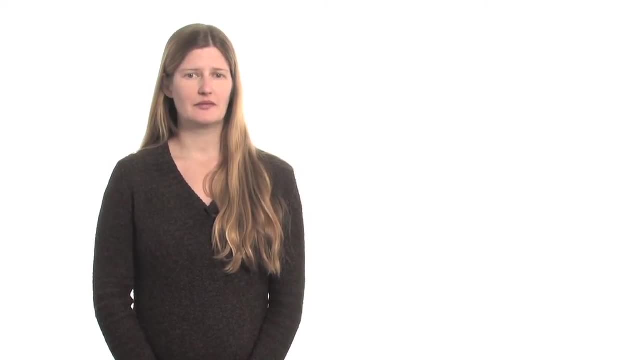 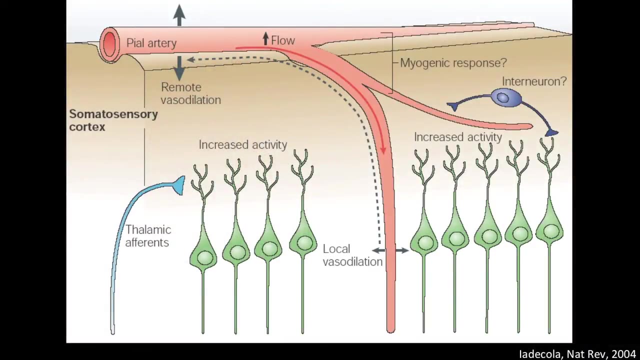 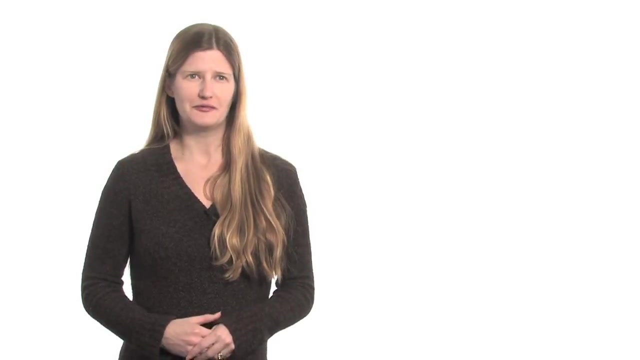 understand blood flow in the brain, And it's very challenging to understand blood flow in any kind of system that doesn't have blood flow, which means that we really need to do this in the living brain, the intact living brain. There are rare opportunities to do. 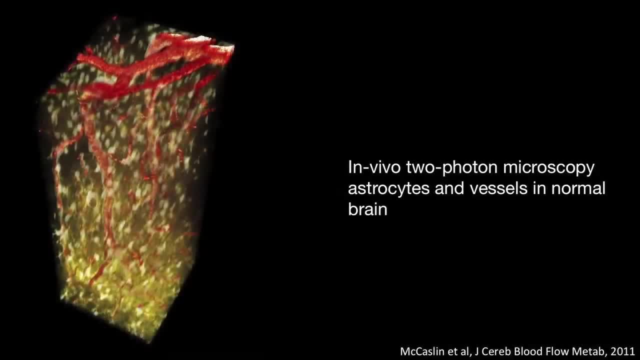 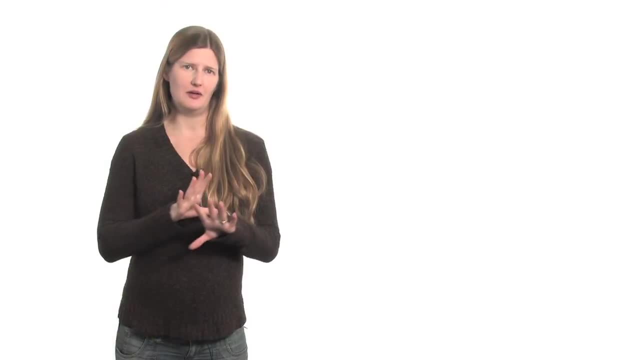 that in humans, and so we very often use animal models. Initially. a lot of the work that we did is we wanted to observe the brain. We wanted to just really get in there and measure as many things as we could at once in parallel to see what was happening, especially when you stimulate the 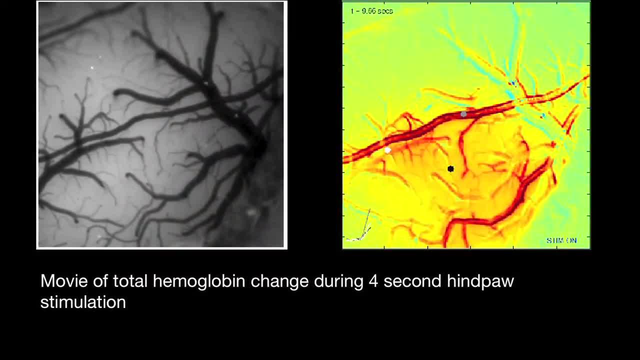 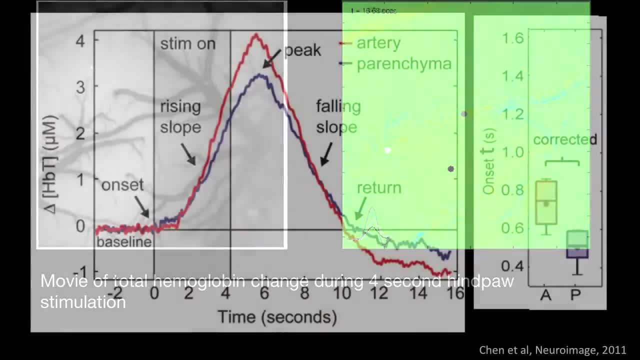 hand, you see an increase in blood flow in a region of the brain And we wanted to really map out exactly what was happening there in terms of all the cells and all of the vessels. But then you get to a point where you're able to build a model and actually say: well, we 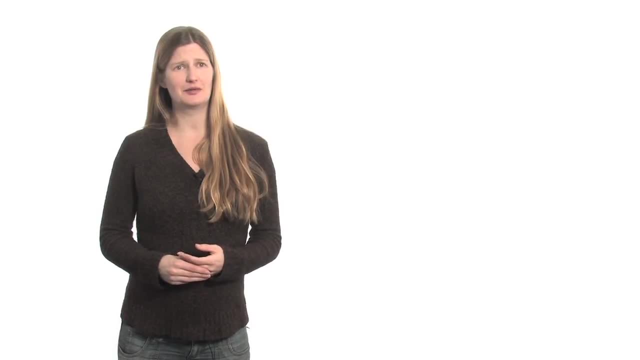 think we understand how this happens, And the only way you can prove that is to be able to actually then modify it in some way or change it, And so that's got us really interested in techniques that can actually affect change in the brain or in tissues, to then perturb something or test something or 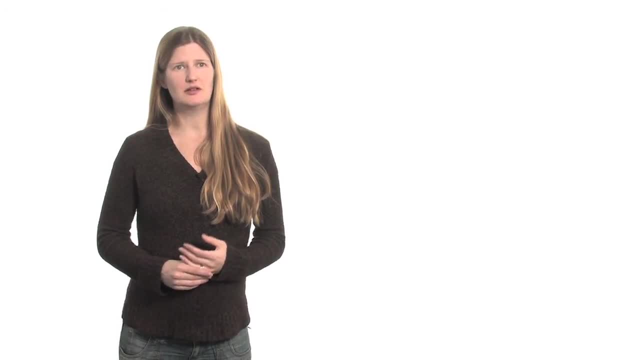 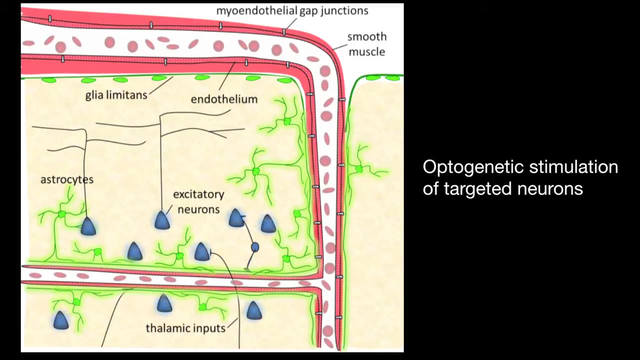 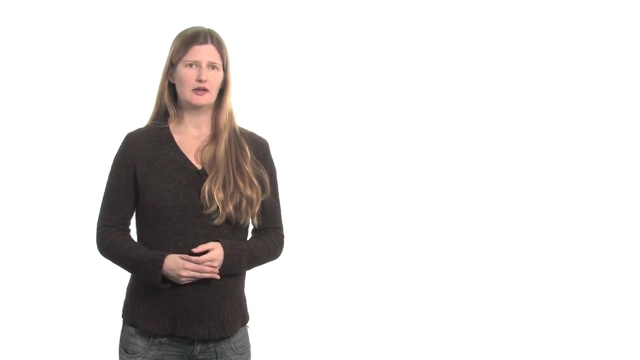 block something, And one new, very exciting technology that's able to do that is optogenetics. So optogenetics is where you introduce this transgenic mutation to a particular cell. that's a cell type which is genetically targeted and allows the cell to express a light-sensitive. 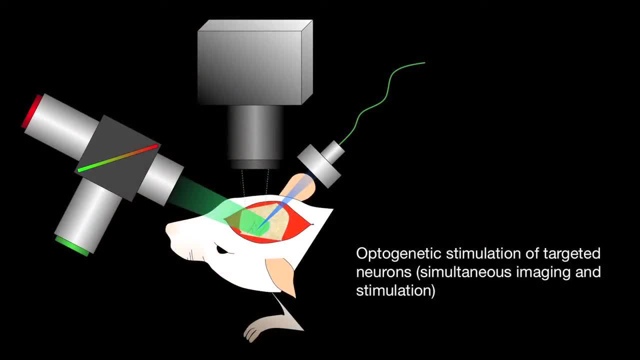 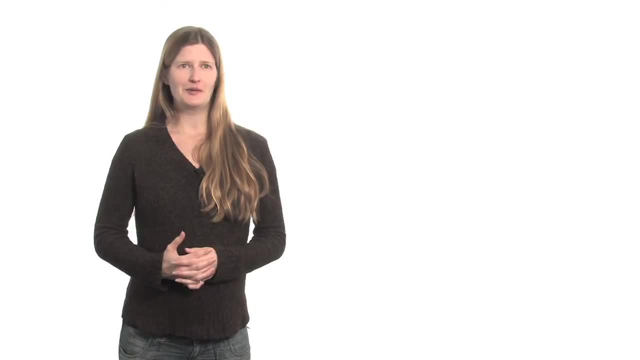 channel, And that channel can either cause the cells to be excited when you shine light on them, or you can cause them to be inhibited, and no doubt you would cause them to do all sorts of other things as well. And so this means that we can say: take an animal use. 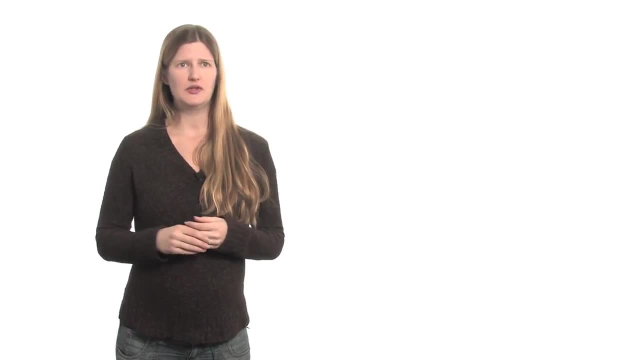 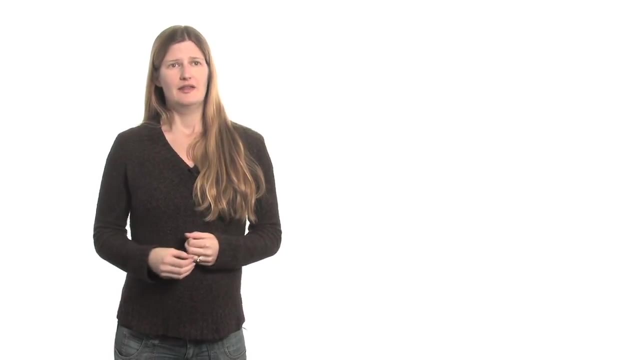 a viral vector to cause this transgenic mutation in a subset of particular kinds of neurons, and then we use light itself To actually stimulate those cells. then we also use light to image the brain to understand what happens as a result of that. But what's really nice is we can sort of use all of those. 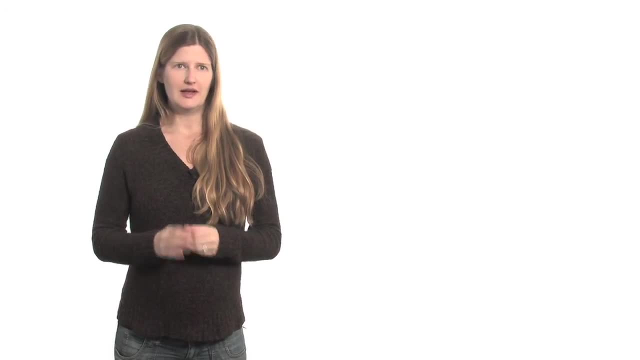 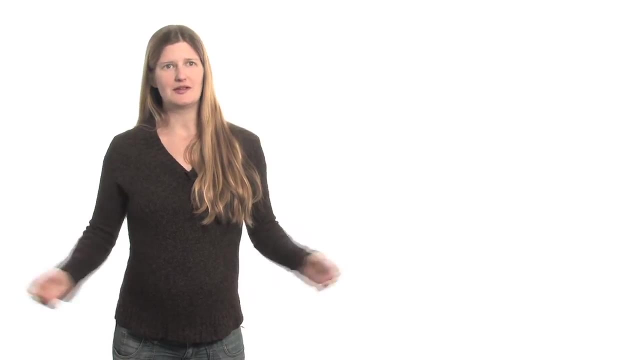 systems together and incorporate them together, and you really get to see what happens at that moment when you turn that cell on and what happens in the subsequent 10, 15, 20 seconds, And so it's a really versatile technique that we can then use to look at other cell. 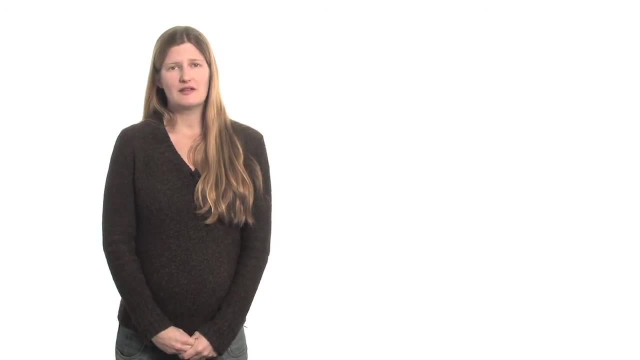 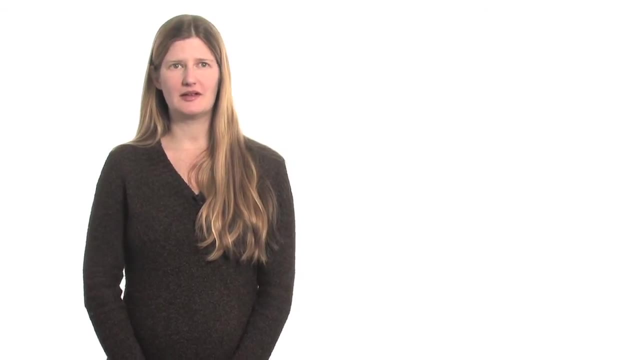 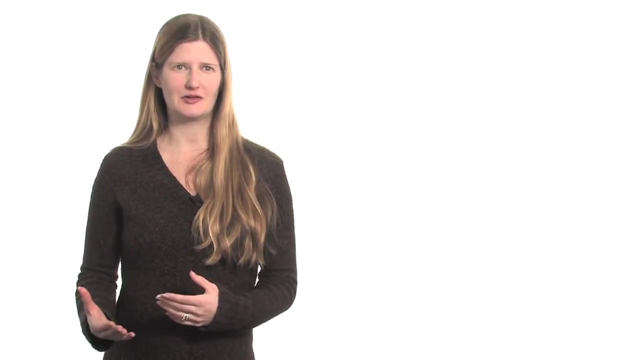 types and other kind of things. And there's other techniques besides optogenetics. Well, there's infrared stimulation of the brain. It's kind of an organic process. Sometimes we see something that sort of stimulates an interest and then it grows from there And 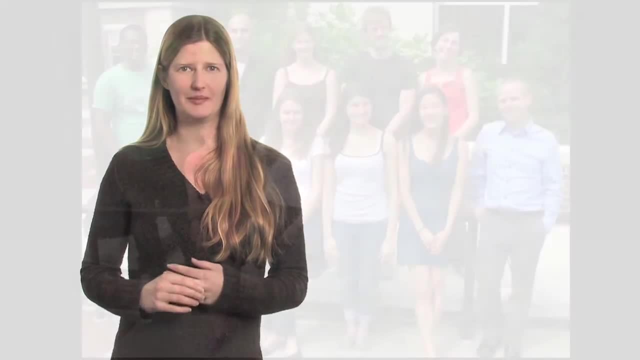 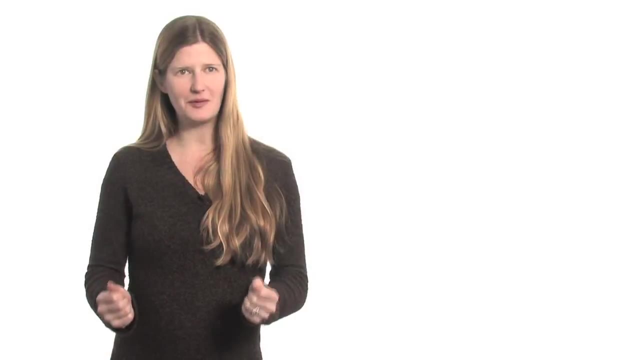 I have a lot of fantastic grad students and postdocs and other people in the lab who have great imaginations as well and who will come to me with a paper and say I think what we have could do something here. So it's interesting.